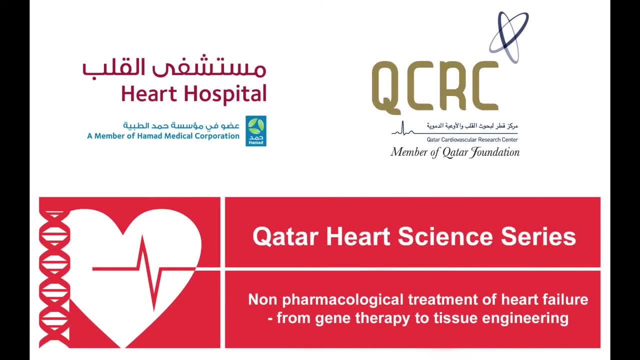 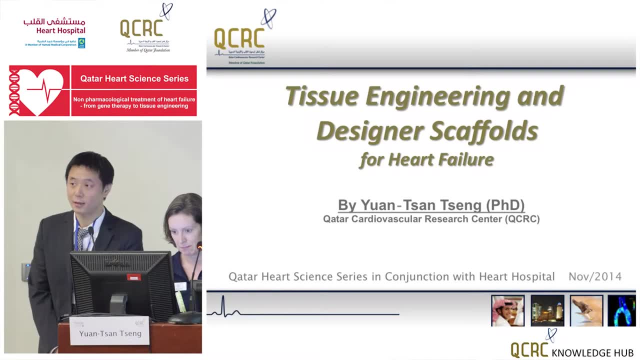 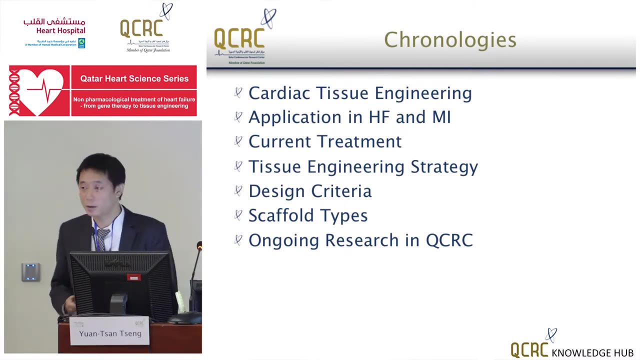 Thank you for a very kind introduction from professor Yacoub, and my talks will be mainly focusing on tissue engineering and especially on the scuffles works. so in application for half ideas, So my my talks will start with a bit of an introduction about tissue engineering and especially for cardiac 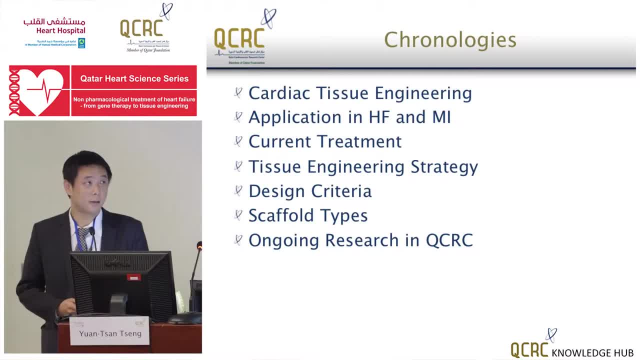 applications and what are the application in the heart failure and especially in myocardial infarctions? and well, audience probably more experienced and I do our current treatments, so I might skip some of those. and what are the tissue engineering strategies for treating myocardial infarctions and what are the 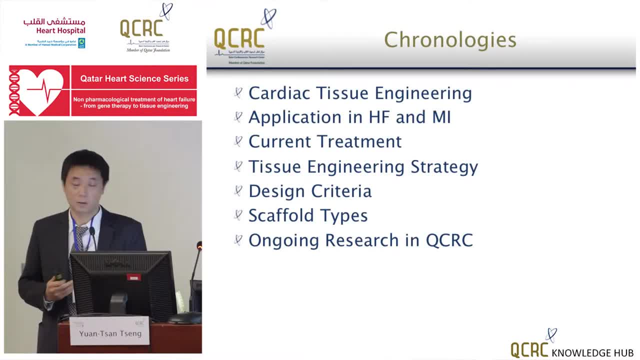 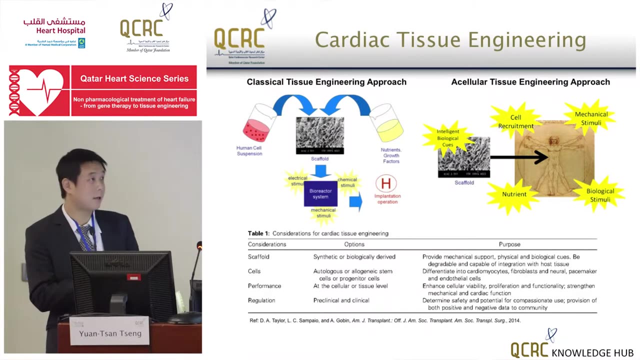 decide criteria for making the scuffles for the applications and what are the current scuffle types currently used employed in tissue engineering and some of our ongoing research in QCLCs. So, in terms of tissue engineering, central tissue engineering, we have the scaffolds. 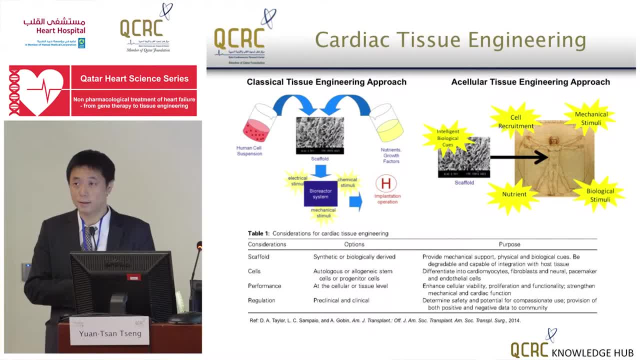 which are the three-dimensional matrix acting as a temporary support for growing cells, and with the nutrients, and follow on with the scaffolds we can put into a bioreactor system to give appropriate electrical, physical, mechanical and chemical stimulation, and followed by implantations of tissue engineering constructs. 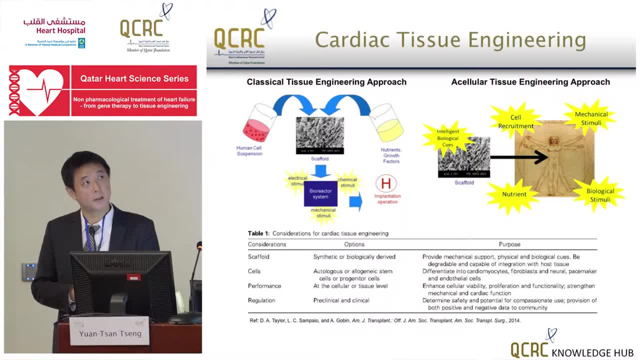 And that's one of our classical approaches in tissue engineering. With the newer approach we are looking at the intelligent scaffolds, where with a cellular approach, so we design the scaffold to have appropriate biochemical signals and actually also physical cues as well- Then we implant direct into humans. 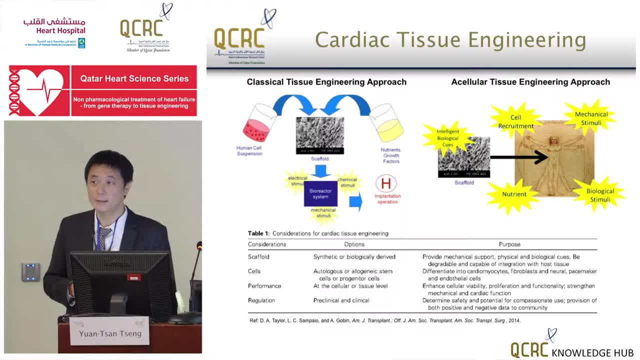 Using humans essentially as the bioreactors and through humans we do cell recruitment and getting nutrients and all the mechanical, biomechanical, biochemical stimuli from human therapy. So one of the main considerations in the tissue engineering, as I mentioned, is the scaffolds and this supports in terms of mechanical, physical and biological cues. 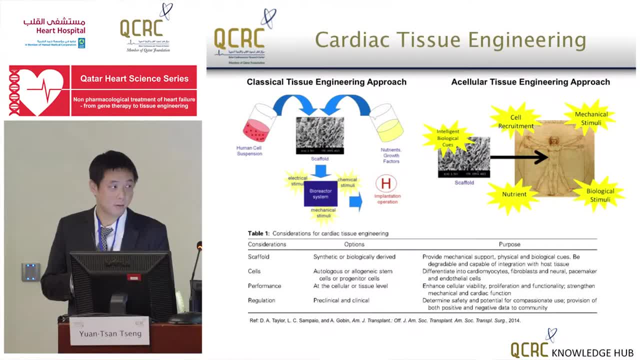 And cells, as we have heard from our colleagues, are very important in tissue engineering. So in our previous talks of Pfizer and Profecia Coov, there are various type of stem cells and actually, Dr Miller, and the stem cells are orthologs or progenitors or IPS, and these 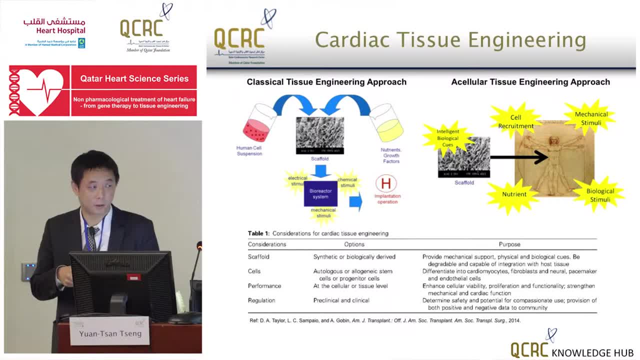 are considered as appropriate cell source. We had to decide which one we want to use And obviously the scaffold performance, both at the cellular or tissue level, is important. So we have to make sure these scaffolds support all the viability proliferations and also 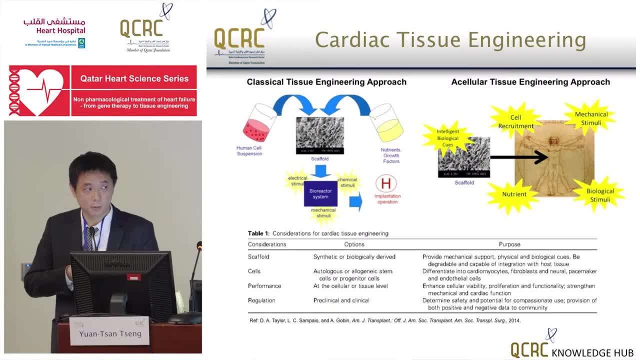 function, such as a support for cardiac functions and mechanical function in terms of the valves. One important aspect in tissue engineering is also regulations, and this regulations has been quite hindrance to tissue engineering developments, where safety and the clinical trial on tissue engineering is very limited and most of it is in 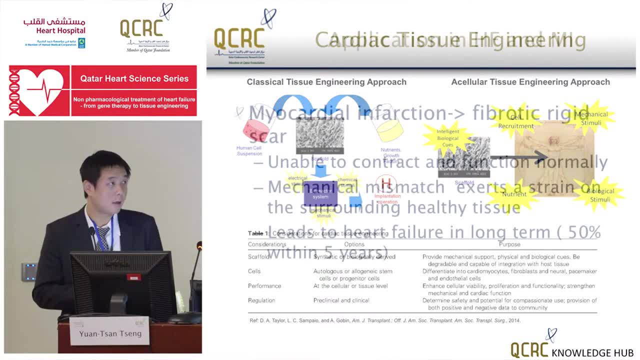 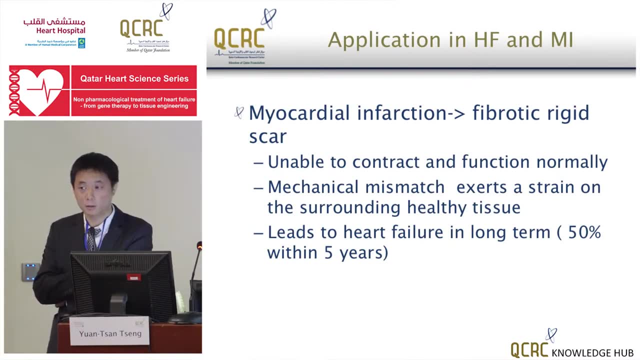 compassionate use. So, as we know, myocardial infarctions generally cause fibrotic collagenous rigid tissues and this effect the function of cardiac cardiac functions. so we all know this. I'll skip this and the current treatments. as Dr Miller has mentioned in the previous talk, use of LVAD and in very severe cases. 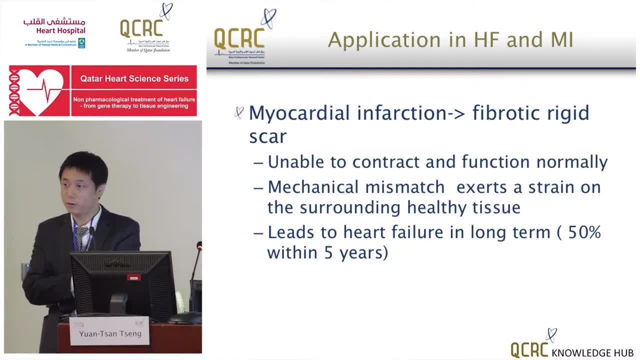 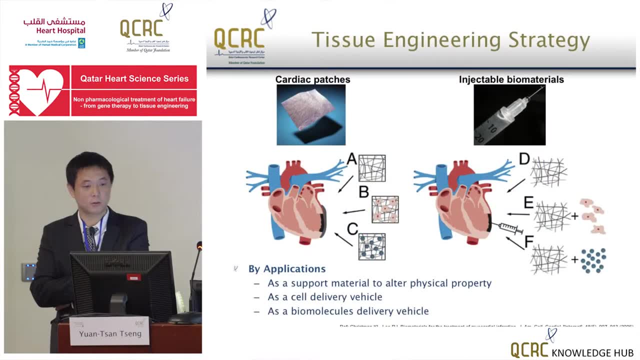 heart transplantations And similar to tissue engineering. we aim to restore or repair the left ventricular functions. So what are the current tissue engineering strategies? We have the use of a cardiac patch or full graft and or use of injectable biomaterials, and these are mainly with three. 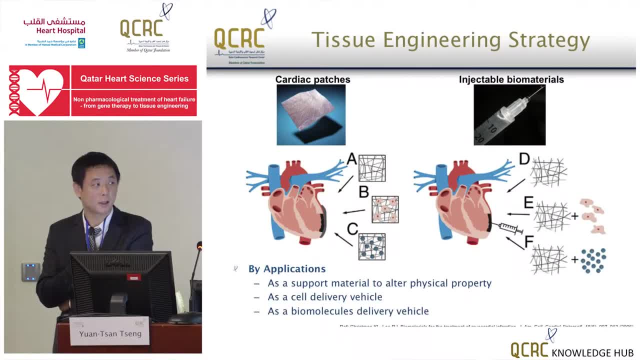 applications in mind, As you can add as a supporting materials. they're ready with the use of a scaffold or the biomaterials. or you can use the injectable biomaterials, or you can use the injectable biomaterials or you can use as a still delivery vehicles. You can deliver stem cells, cardiomyocytes and 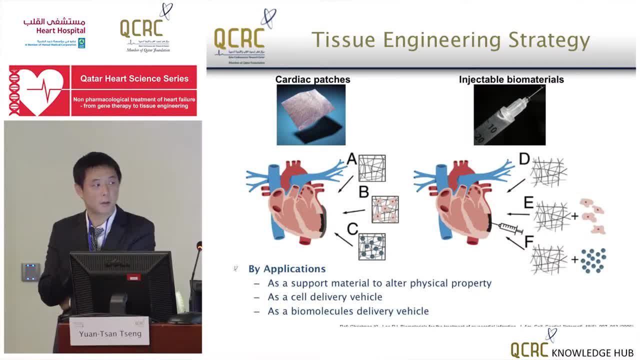 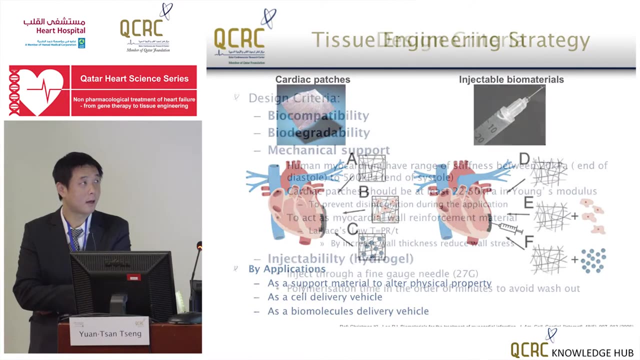 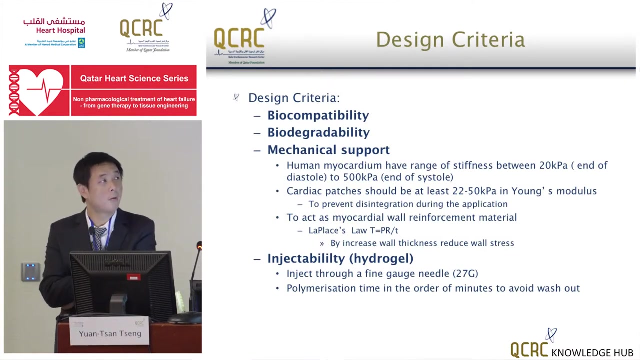 depends on the choices. or we can use as a biomolecule delivery vehicles, So it could be a mRNA, as mentioned by Dr Spina yesterday's gene therapies, and or refractors, etc. So, with this application in mind, what are the criterias we need to think about when making the scaffolds We have? 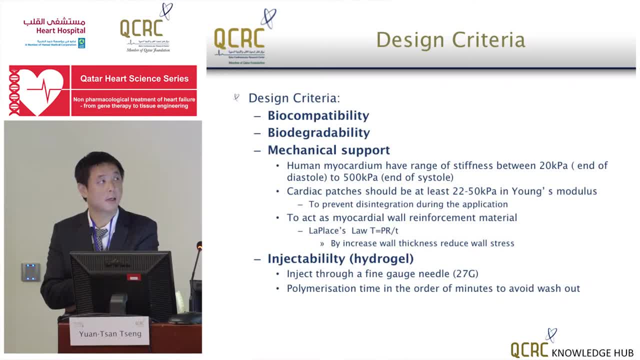 the thinking about biocompatibility and about degradability. These are important where the polymers that we implant has to be non-toxic, non-eugenic and, in relation with the degradation, is degradation product has to be non-toxic as well And, in addition, 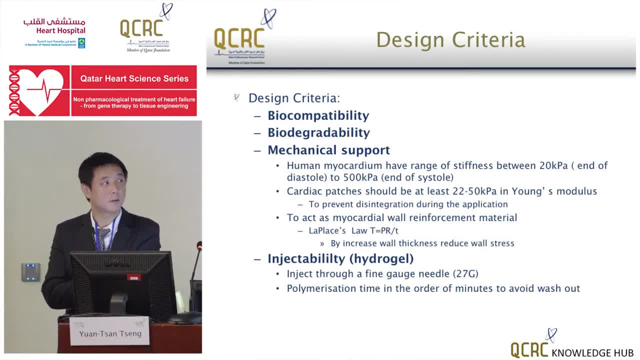 to the polymer property itself. we also need to think about mechanical support. When you have a human myocardial, we have stiffness between 20 kilopascals to 500 kilopascals and if you are thinking as a cardiac patches, for example, molecular delivery vehicles we need. to have this some stiffness. so generally we consider 20 kilopascals to make sure the patches stay there. And if you have application in mind where you are using as a reinforcement material for myocardial walls, we need to consider where. what are the stiffening factors? what? 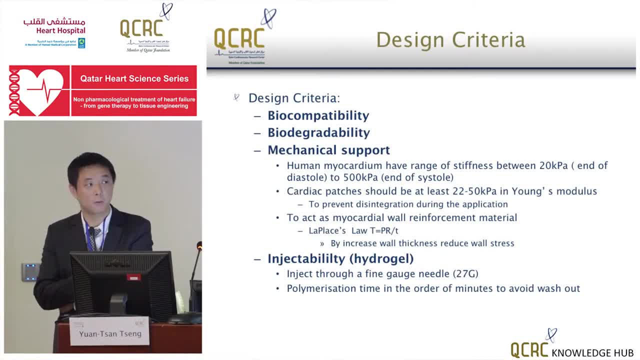 stiffness, you need to support the wall, to reduce the wall stress. And in terms of hydrogel application, where the injectable biomaterials, you need to consider things like the gels has to be able to go through the needles used for injections and while the polymerization 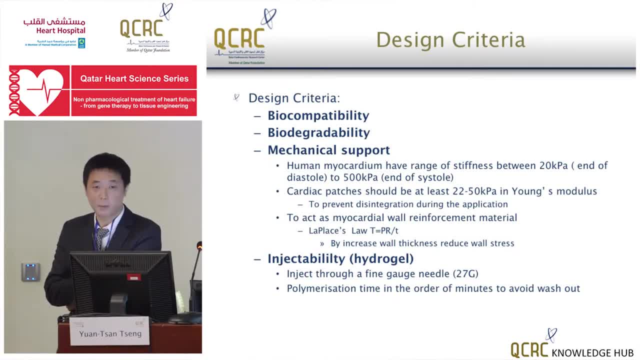 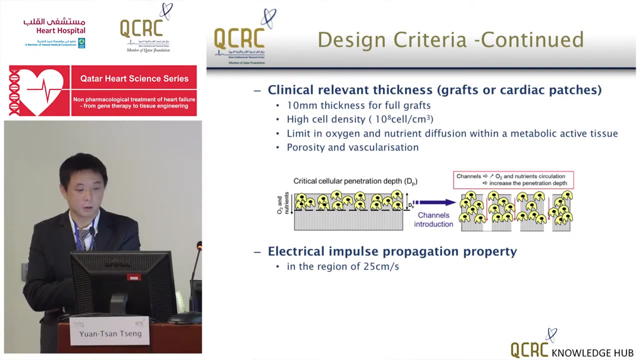 time from the solution to gels. that has to be timing right so that you can actually inject the materials, but at the same time, it has to polymerize in time so it doesn't get washed out. In terms of using grafts or cardiac patches, you have important criteria as thickness. 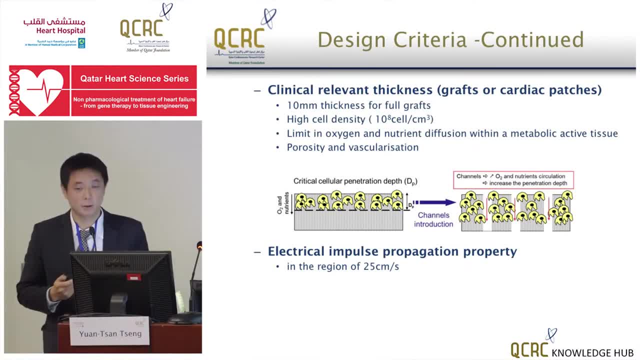 So if you consider, for example, full grafts, generally we are talking about 10 mm thickness and cardiac tissues are very high cell densities and has a very high metabolic rate. so you will run into what we call diffusion constraints, where the oxygen and nutrient diffusions are. 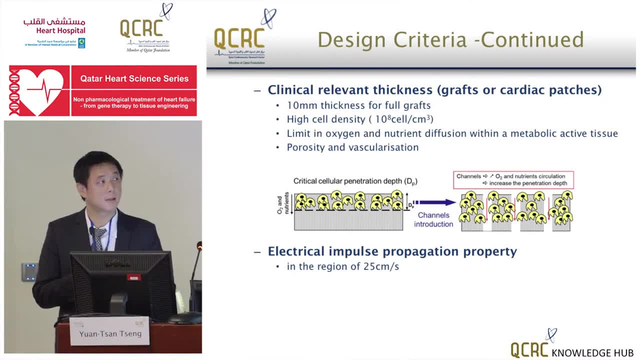 limited. So one of the strategies people consider is taking care of the porosity and vascularization where you introduce channels, essentially like blood vessels, to actually enhance the cell polarization and colonization into a full graft And especially for cardiac tissue engineering. one important aspect is thinking about electrical impulse propagation. 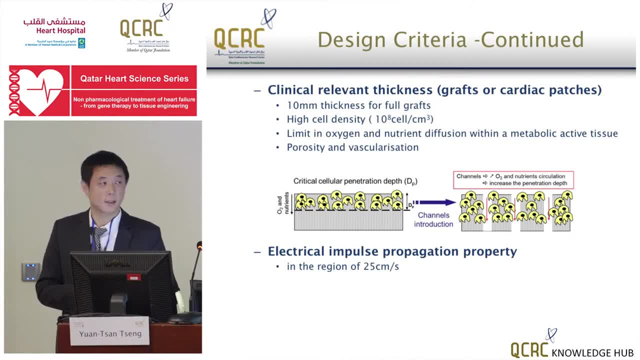 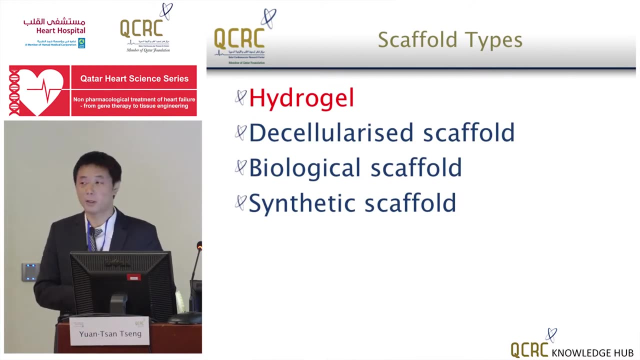 rate. So we know that cardiac tissues have taken electrical signals, so we need to consider this as part of the design criteria. So, with this in mind, let's look into the four common scaffold types that are currently used in tissue engineering. These are hydrogels: decellularized. 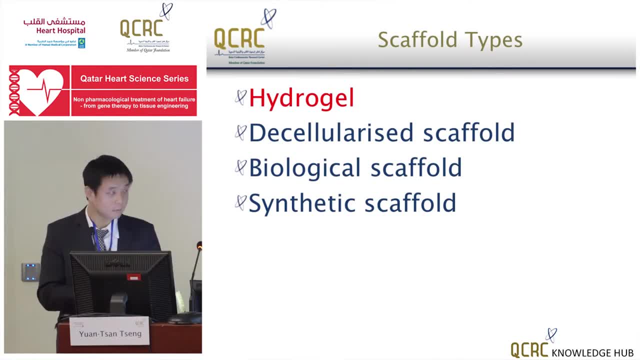 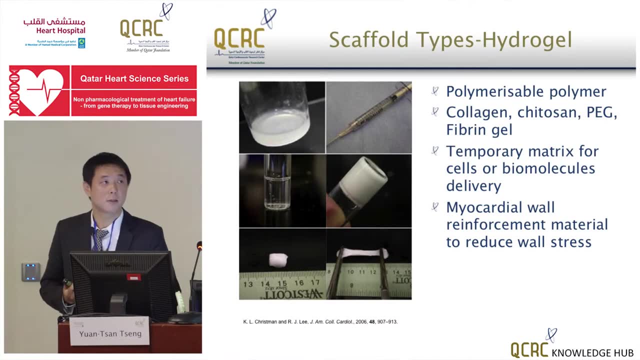 scaffold, biological scaffold and synthetic scaffold. The hydrogels generally are polymerized for polymers made from either collagen, ketosan, polyethylene glycane or fibrin gels- And this you can have clear solutions and then generally polymerized. 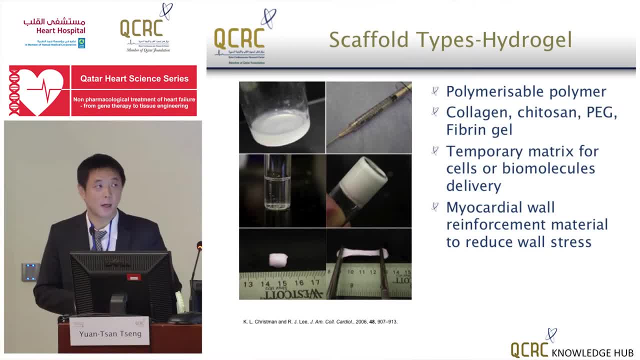 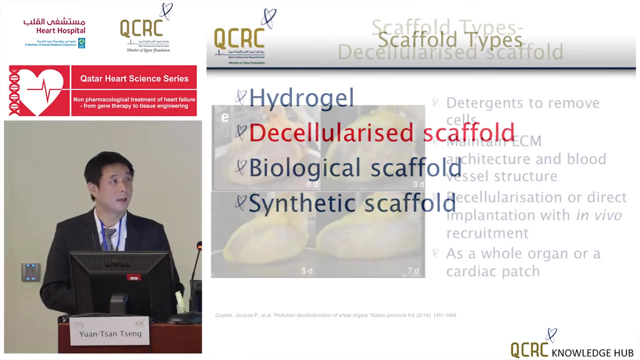 And this mainly acts as a temporary matrix for cells or biomolecular deliveries. And you could also add myocardial wall reinforcement, where some of the gels actually can be designed to have a very good stretch, stiffness and mechanical properties. And the second type of scaffold I'm going to introduce will be decellularized scaffold, And these are scaffolds. 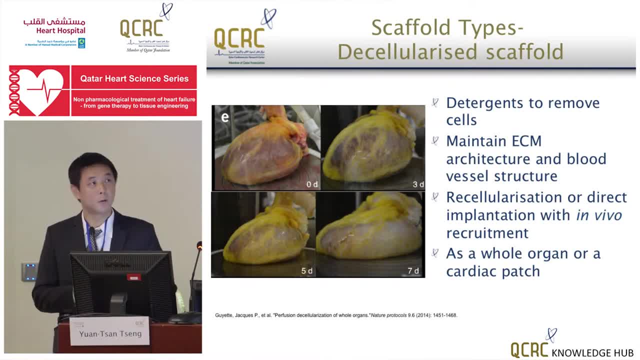 taken from a whole organ or tissues And then we remove the cells via detergents And you can see in this heart where there's a protocol, where people decellularize a whole heart over seven day periods, where you can see the red where the cells are being removed and you're left with essentially like a collagenous. 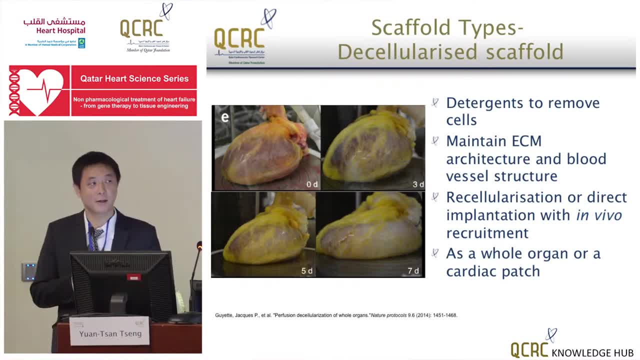 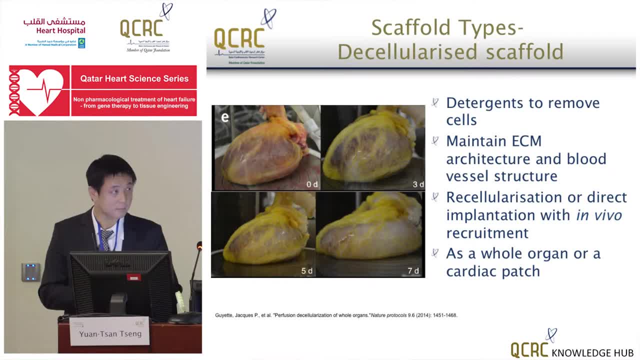 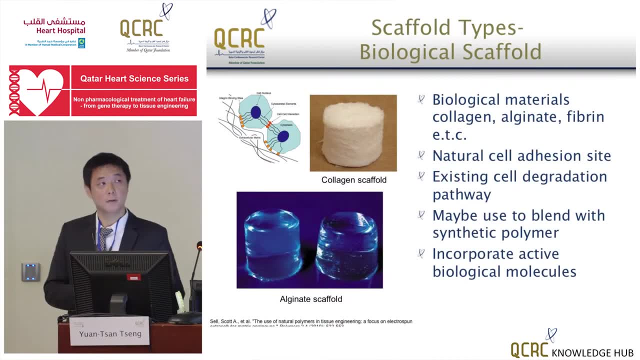 good way to do it. So this is a very good way to do it. So this is a very good way to do to involve a recruitment. and third type of scaffolds i'm going to be discussing about is a biological scaffold. so biological scaffolds are material that is biological in origins. 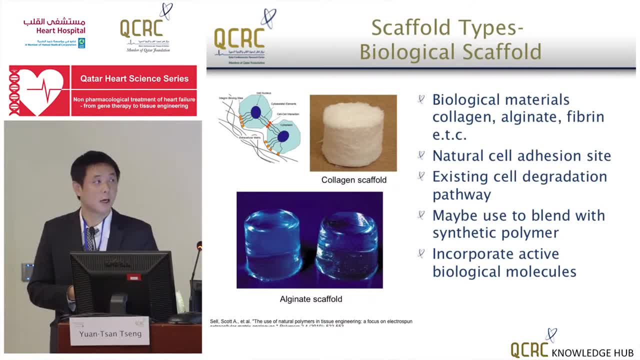 so these are collagen, alginate, fibrins and etc. and they have advantage where it has natural adhesion cell size and its degradation pathway is actually existing most of cells already. so it's often used to blend with other synthetic polymers, which lacks of a natural adhesion size and can be over cooperated with other biological molecules as well. 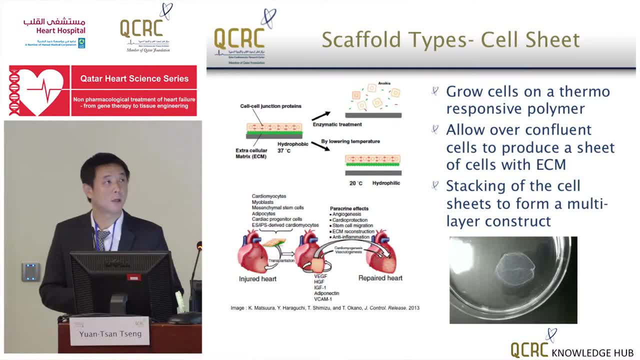 so one interesting type of natural biological scaffolds is the use of cell sheets- which i believe is also in our previous seminars- where they grow cells on a thermal responsive polymers and the cells will become conference and produce adjacent matrix and by the special property of this type of polymers, when you change the temperatures it actually 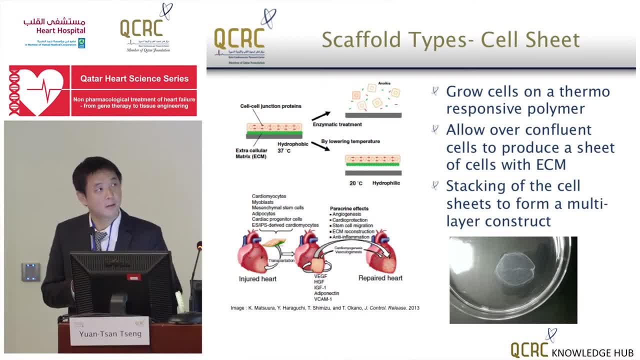 becomes hydrophobic to hydrophilic, which allows the cell to detach and this you can see a detached cell sheet like protein and pbs solutions. so essentially you have a sheet of cells with the extracellular matrix intact and this has a potential application where we can use for 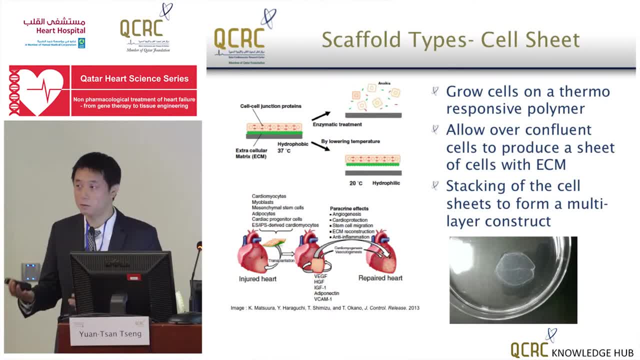 transplantation to injure hearts, and by introducing the right cells we might be introducing a right pyroclastic effect as well, and it's also possible to use the same type of cell sheet for multi-layer constructs. of course, there are problems with the mechanical properties in this aspect, and the last type of scaffold i will introduce is: 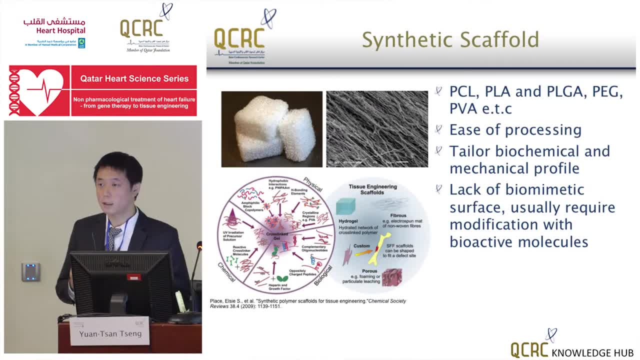 synthetic based scaffolds, and these are scaffold made of synthetic biomaterials which are, for example, polycarbonate, electron, polylactic acid, peg and pva, for example, and they have advantage where it's actually very fairly easier to process and lots of existing processing factors exist and you can tailor its biomechanical profile or about chemical profile by using. 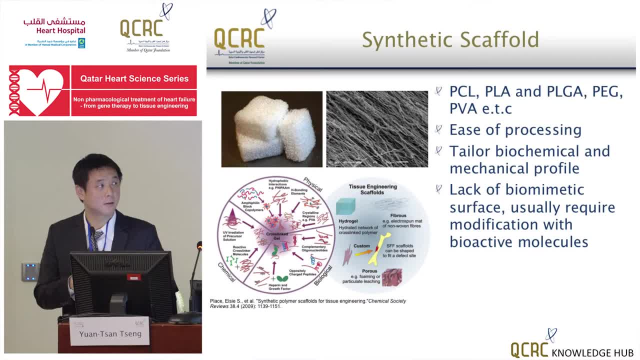 either pros, nanofibers, or by introducing different physical properties, chemical properties or by introducing biological signals into the scaffolds as well, and there are different type of forms where you have gels, fibers, you can do soil free fabrications or you can make a porous scaffold like this type and general synthetic scaffold. lack of 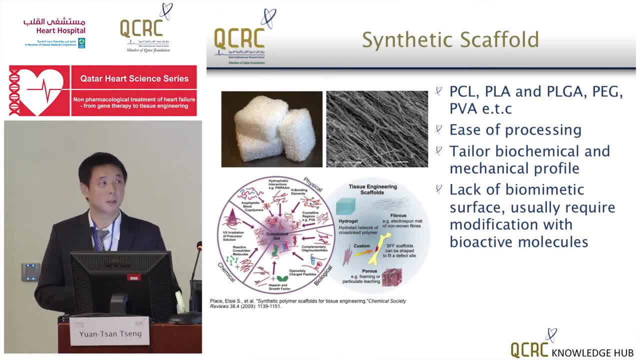 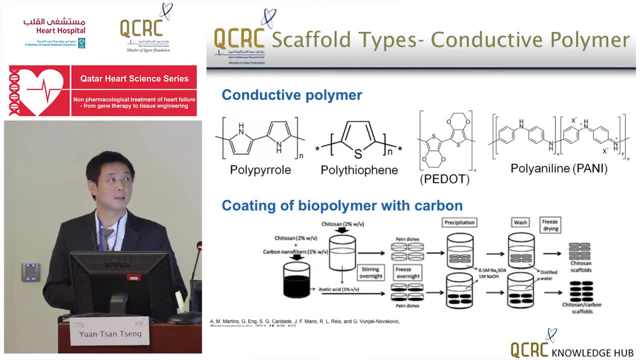 biomimetic surface, but so we usually cooperate with some sort of biological molecules, and one type of synthetic scaffolds or synthetic polymers are interesting in cardiac tissue engineering and especially in neural tissue engineering as well, is use of conductive polymers, and these are special type of polymers with loose pi electron systems, where 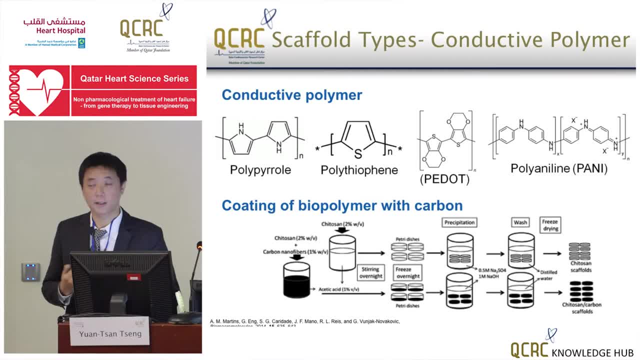 they act like a metal, so it actually provide conductivities and so you can use this polymer directly. or another approach is actually taking existing biopolymers that we use, such as ketosans and silk in one of the reports that you can coat it with something electroconductive. 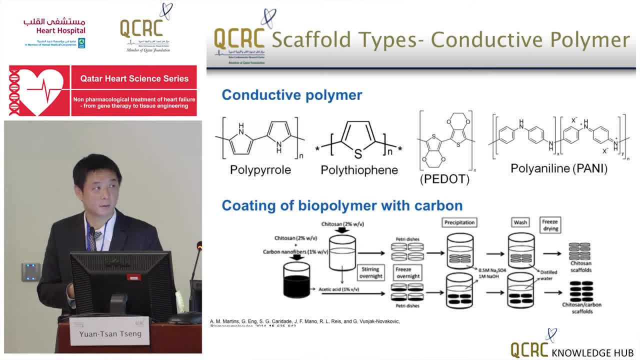 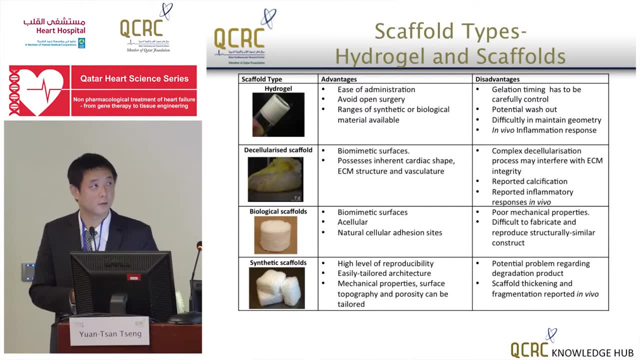 so, such as carbons, and this actually provides similar properties as well. so this is a quick summary about advantage and disadvantage of using different type of scaffold. it really depends on the applications of the materials. so, such as hydrogels, you can use because it's easier. 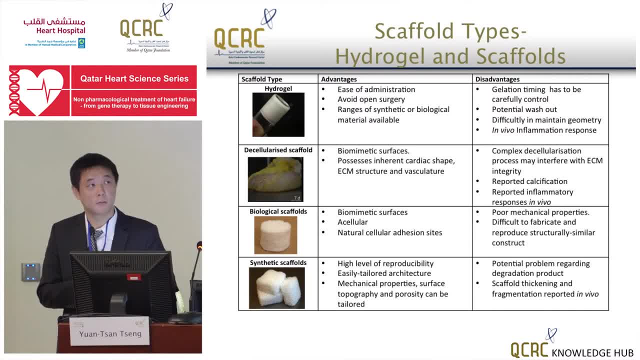 to administrate. you can avoid open heart surgeries, but the problem is you have the duration times and potential washout you have to be considered and geometry of hydrogel is generally more difficult. Distillerized scaffold is very good because it actually maintains ECM structure and vasculature, but the complication in the distillerization process generally 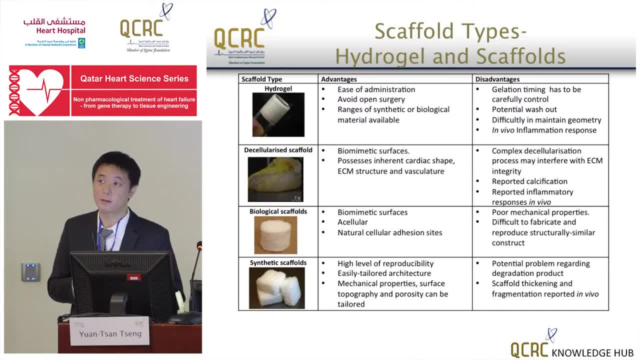 a failure: ECM integrities and maybe there's some incomplete wash so you may get cell depres, which some people believe they cause inflammatory responses or lead to constipation and so on, And biological scaffolds, which are generally very good in biomimetic surface and 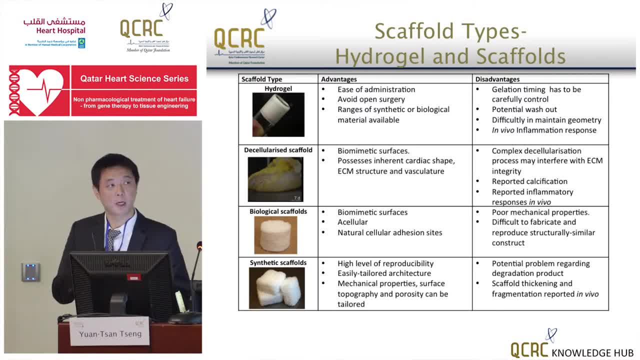 there's no cell exist, but probably poor mechanical properties are often associated with this type of polymers. So this is the end of my presentation, Thank you. So the text scaffold, on the other hand, is very easy to produce and you can tailor the architectural. 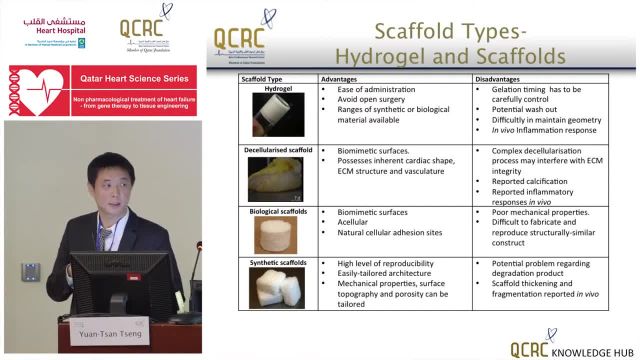 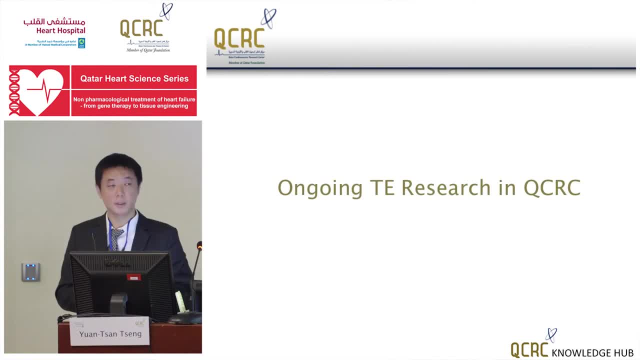 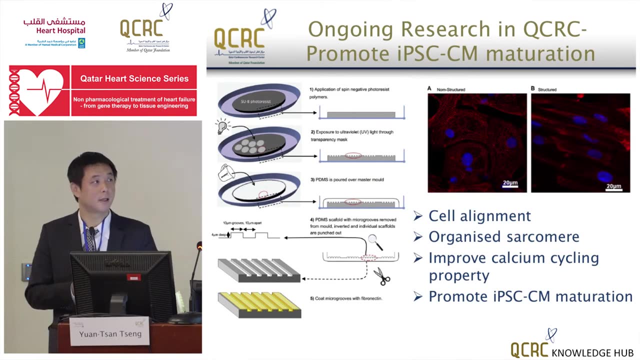 mechanical properties, for examples. But degradation products are always a concern as well, and they are in some studies where thickening and fragmentation of the polymer actually cause some problems. So what are the ongoing research in QCIC, especially in tissue engineering field? One of our previous studies is looking at 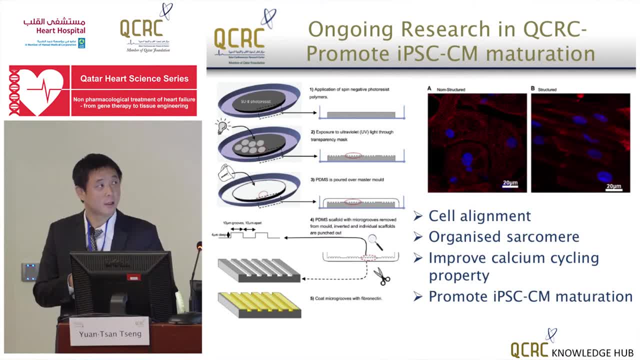 maturing IBSC cardiomyocytes. So, as Professor Yacoub mentioned, we are using physical cues to promote maturation of the immature cardiomyocytes. So the photography is: we actually make a mold with lots of pole, lots of grooves about 10 micrometers apart, and we cut with PDMS and 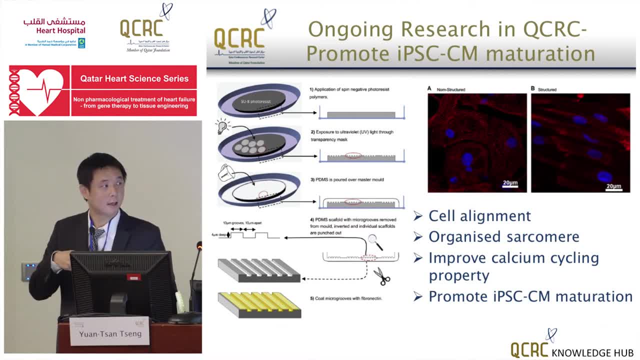 use PDMS as a material for our scaffolds And this allows- oh actually, I'm sorry, a forgot to say then we call it fibronectin- to allow cell adhesion. This allows the cells to actually adhere with the groove and align with the groove. So by providing alignment, 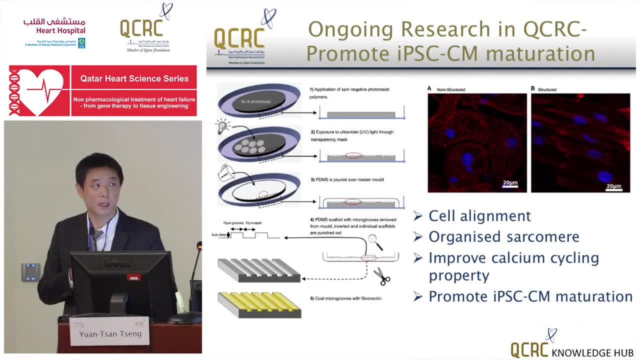 facilities we actually promote the immature type of cardiomyocytes to show cell alignment, organize subcremials and even improve some of the causative signaling properties. So through physical cues we can actually promote IBSC cardiomyocytes, Thank you, And also maturation. So our ongoing research is actually moving to using polycarpolectum. 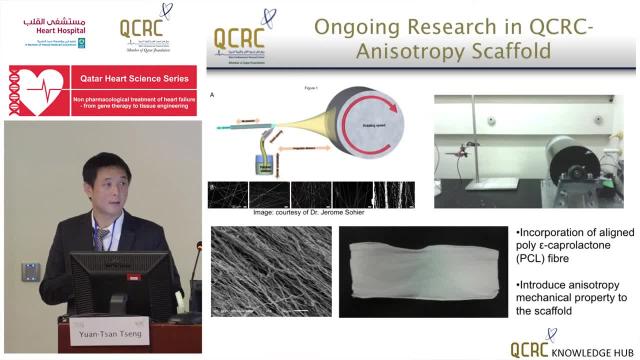 fibers, which are also aligned, and we do this through a jet spraying techniques, where we spray the polymer of PCL in air guns at a very fast rotating speed of the drums. This actually provides alignment. As you can see, we increase the speed of the drum, we increase. 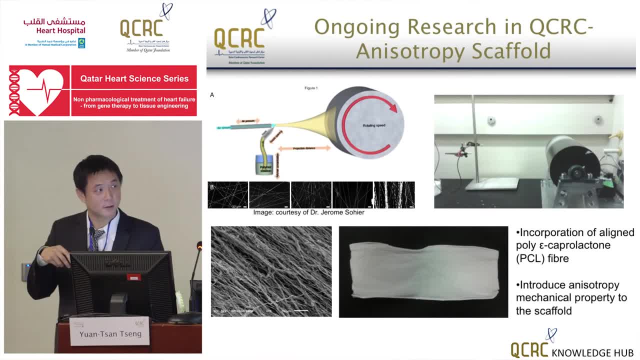 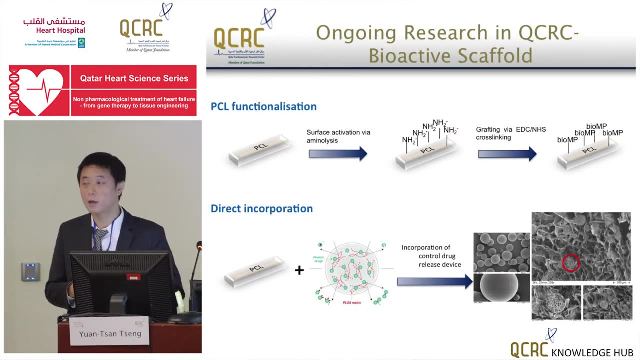 the alignment And this is an actual thick scaffold, so you can see in here- And we introduce both the alignment, allow the cell to align with it and also change the mechanical properties into an antisocial properties as well. And one of the ongoing research as well is modification. 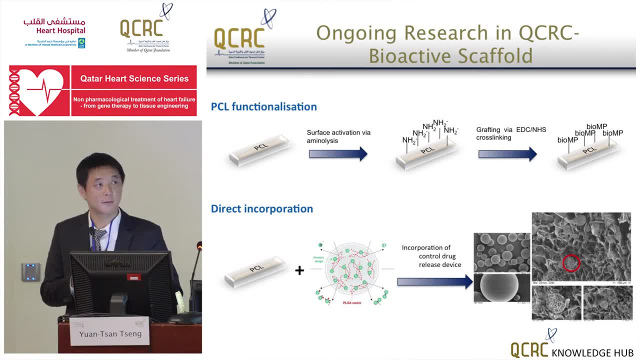 of the PCL itself. So we can either modify the surface with biomimetic molecules or we can incorporate interesting molecules- drugs- into a scaffold. So we can modify the surface with biomimetic molecules or we can incorporate interesting molecules- drugs- into a scaffold. 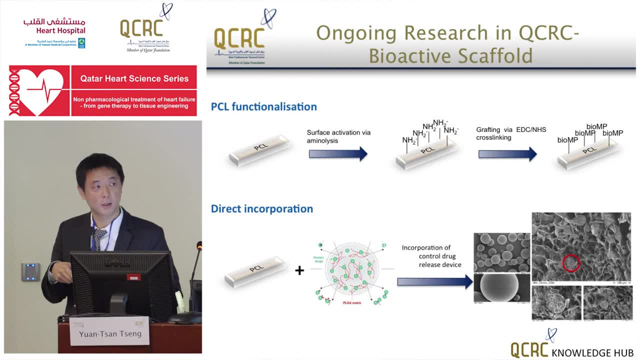 So we can modify the surface with biomimetic molecules, or we can incorporate interesting molecules- drugs- into a scaffold. So we can modify this into a some sort of drug related devices that we incorporate into the scaffold as well and then provide a long-term and local release of the drugs or growth factor. 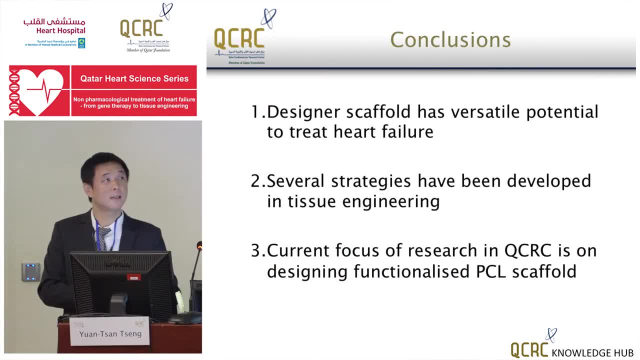 proteins. So, in conclusion, the standard scaffold has very versatile potential for half radius treatments And there are several strategies that have been developed in tissue engineering. old strategies are being considered. they all have its advantages and disadvantages, So this is a lot of ongoing research focusing on this. 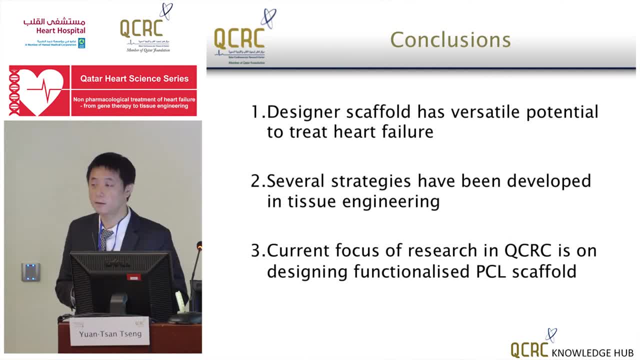 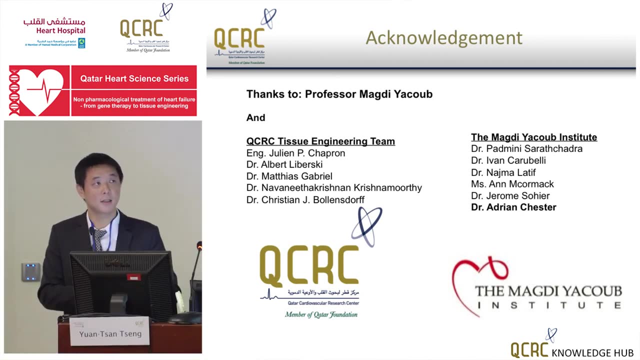 research focus on this And in QCLC we mainly focus on designing functionalized PCL scalpels and in applications for treatments. And last slide- long term- is thanks to Professor Koop and our teacher engineering team in QCLC and our team in London in Magyar Koop Institute. Thank you.